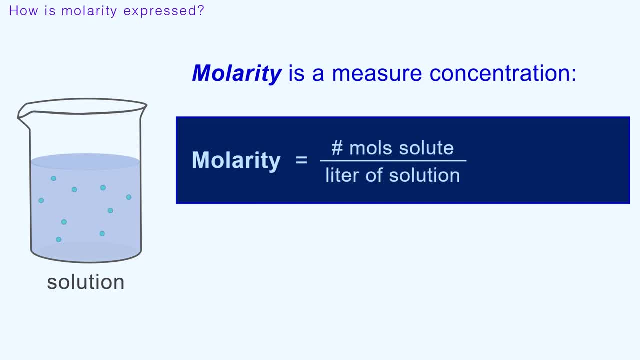 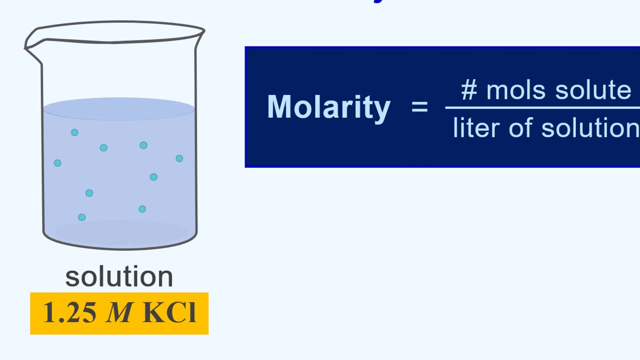 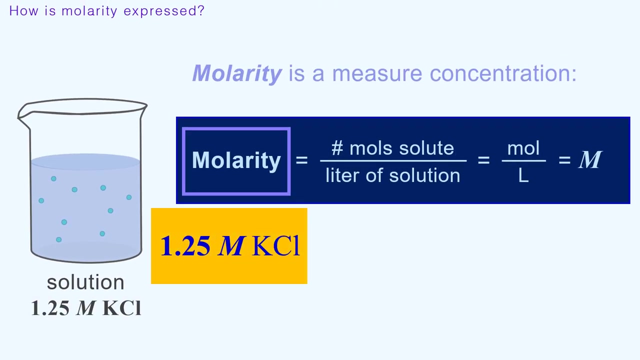 is the number of moles of solute divided by liters of solution, expressed as moles per liter and symbolized with a capital M, sometimes italicized, which is pronounced molar, Molar. Let's say we have a 1.25 molar solution of KCL, So 1.25 is our molarity. 1.25 MOLAR KCL tells us there are 1.25 moles of KCL dissolved. 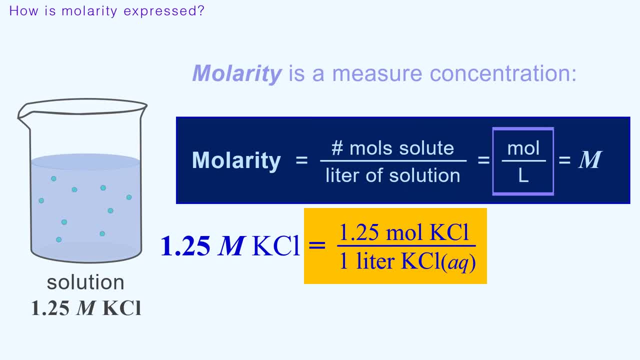 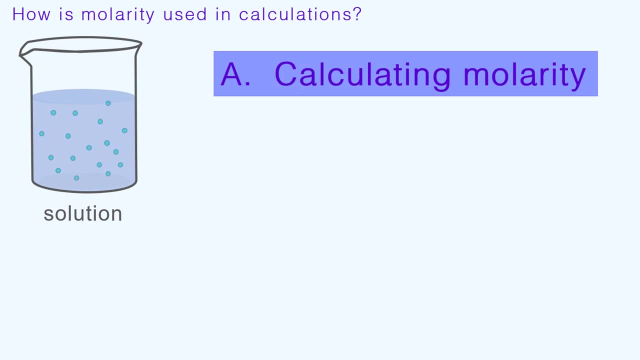 for every 1 liter of solution, or 1.25 moles per liter. 1.25 molar represents 1.25 moles per liter. Let's take a look at how we can use molarity mathematically. First we will look at how molarity is calculated and then use molarity in a calculation. 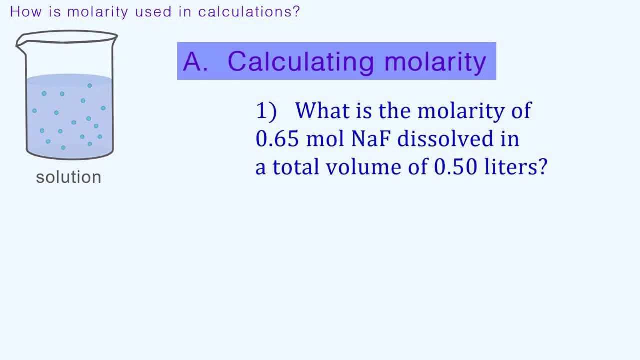 First problem: what is the molarity of 0.65 moles of sodium fluoride dissolved in a total volume of 0.50 liters? Molarity is moles per liter, so we divide 0.65 moles by 0.50 liters of solution. 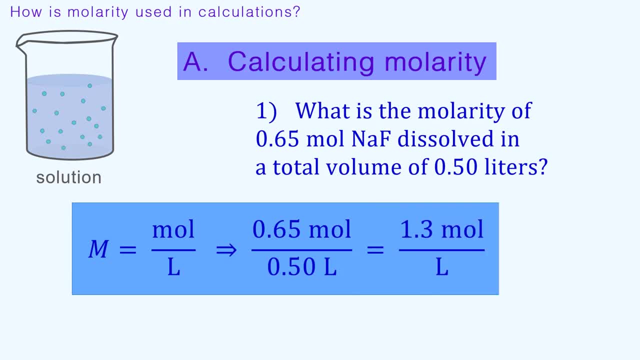 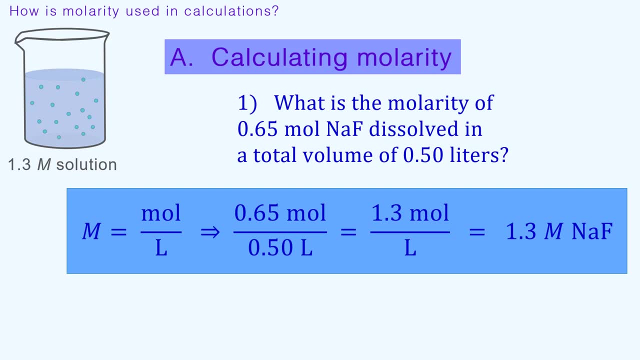 and find the concentration to be 1.3 moles per liter or 1.3 molar sodium fluoride, The molarity is 1.3 molar. Problem number two in which we now have molarity: we now have not moles but grams. 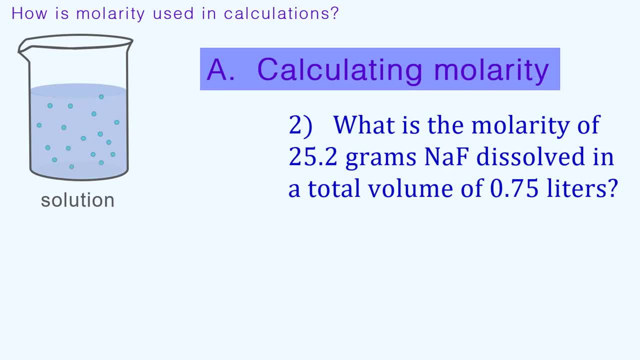 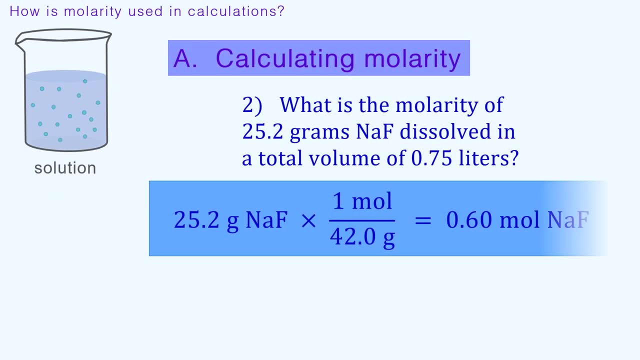 What is the molarity of 25.2 grams of sodium fluoride dissolved in a total volume of 0.75 liters? Since we have grams and not moles, the first step would be to determine the number of moles using the molar mass of sodium fluoride. 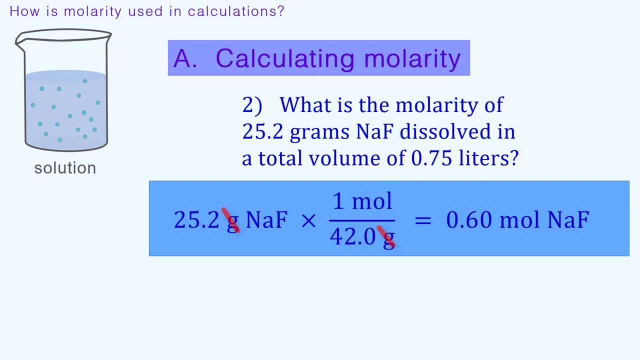 which is 42.0 grams per mole. Here grams cancel and now we have 0.60 moles. sodium fluoride Molarity is moles per liter, so 0.60 moles divided by 0.75 liters. 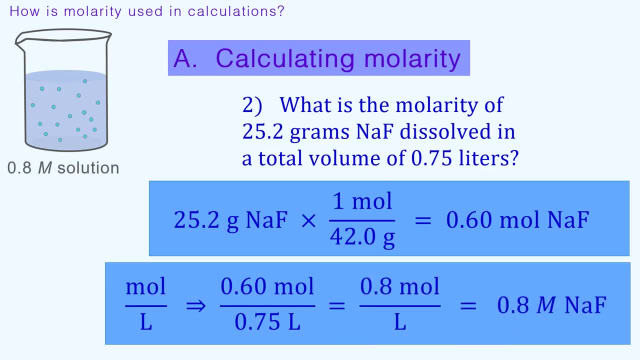 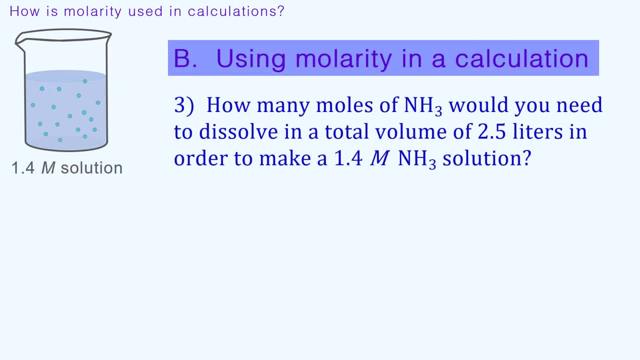 gives us 0.8 molar sodium fluoride. Now two problems to look at using molarity in a calculation. Problem number three asks how many moles of ammonia- NH3, would you need to dissolve in a total volume of 2.5 liters in order to make a 1.4 molar solution?